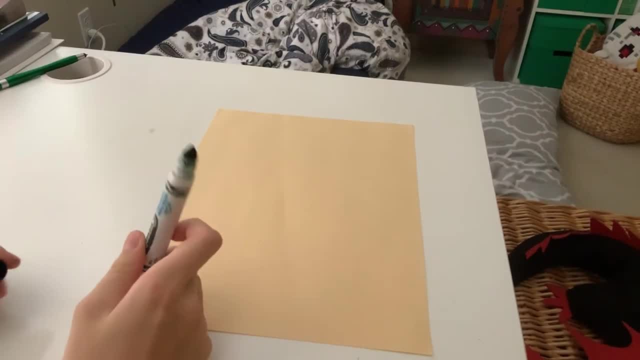 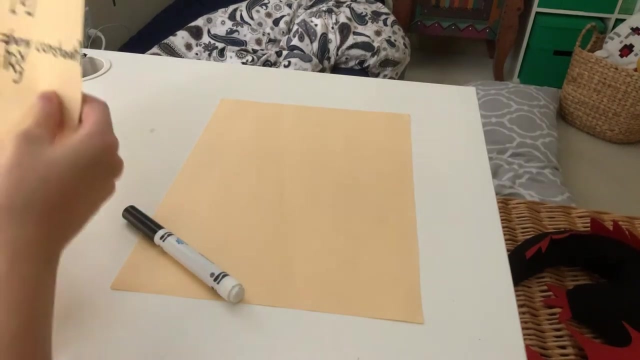 Welcome back everyone. So sorry for missing a day yesterday of recording, but I was a little busy with again all the work that I've been getting and simply because it was a holiday as well. So today we are going to be. you know, it's a little bit of a continuation of the end of the last video, so I just want to briefly take a look at what we did at the end of the last video. 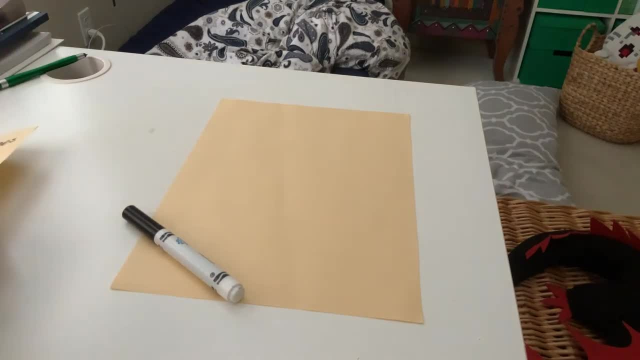 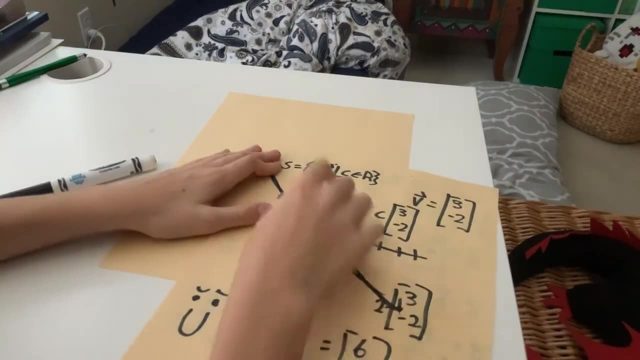 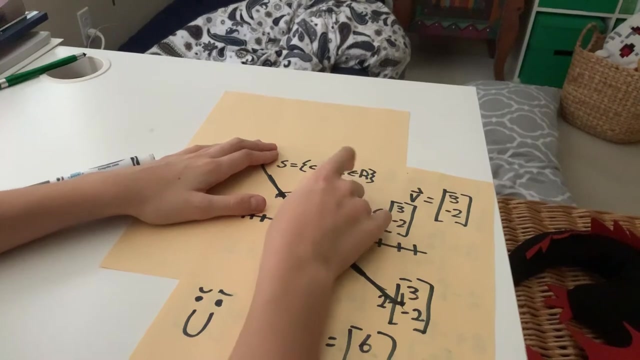 So which page was that? Fairly certain, Here it was. So here we attempted to define a set where we multiply some constant c by some vector v, such that c is actually a constant that is a member of the reals right. 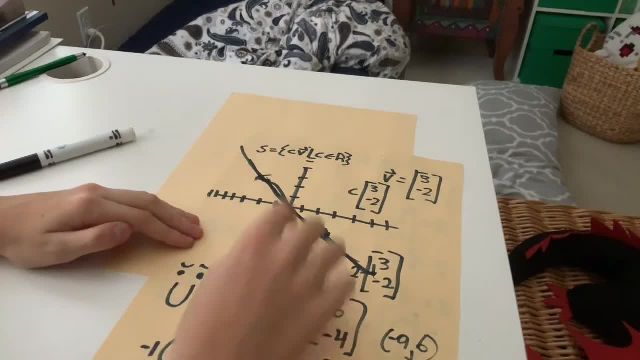 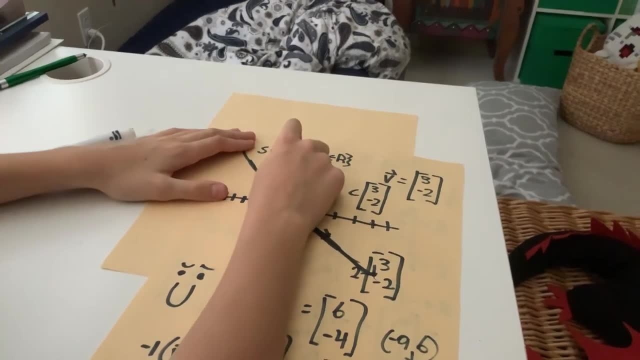 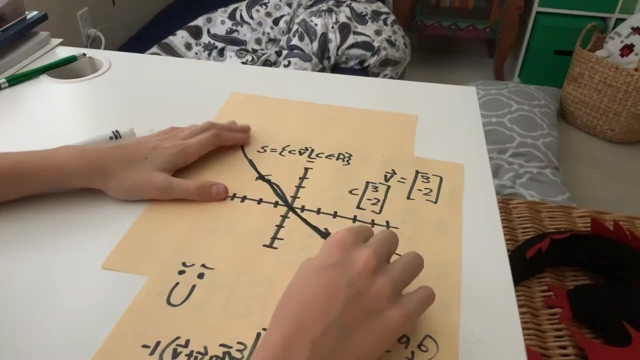 So we defined our set in this way and we said that whatever this v is, whatever its magnitude is- in this case we're saying it's a position, a vector- that any constant multiplied by c in its standard position- that's our specification- it can all be graphed through this line. 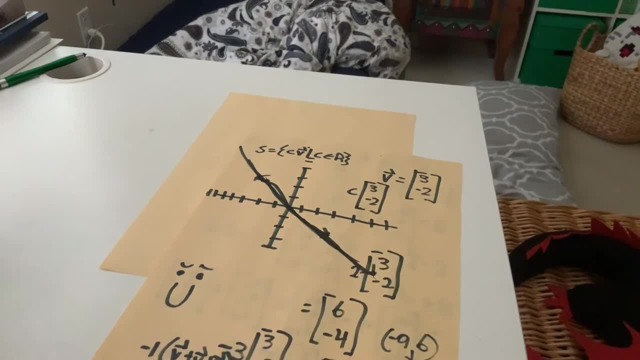 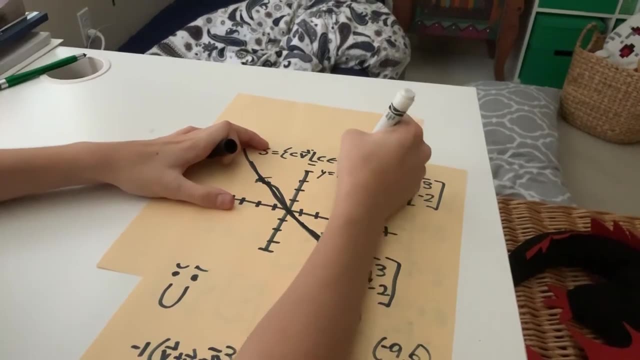 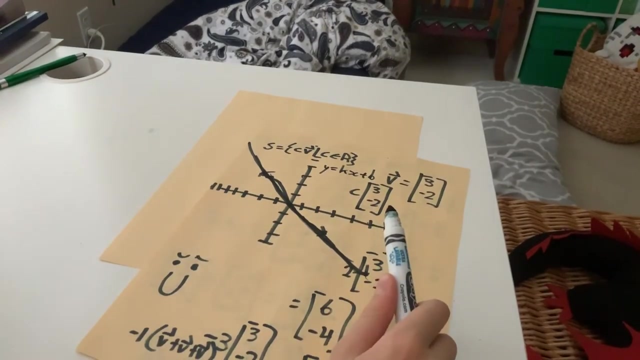 So in essence, it's kind of like this equation: y equals kx plus b, right? In essence, that's really what it is, And you might ask why it has. Why does it have to be so complicated, right? 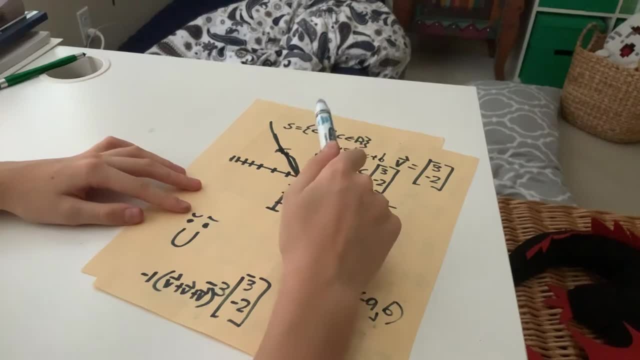 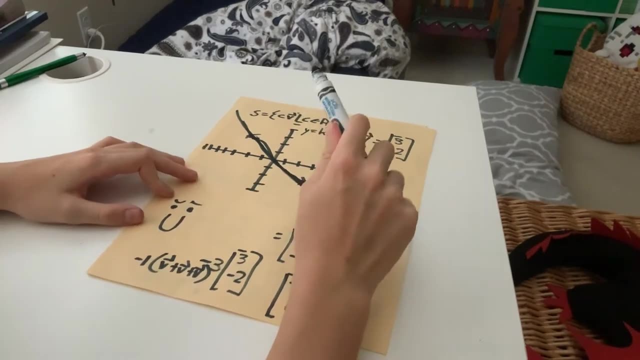 y equals mx or kx plus b is much more simple than the set of this obsolete or obscure set definition that I've given. Well, the reason this is so useful is because it can be used in three dimensions, it can be used in four dimensions, etc. etc. 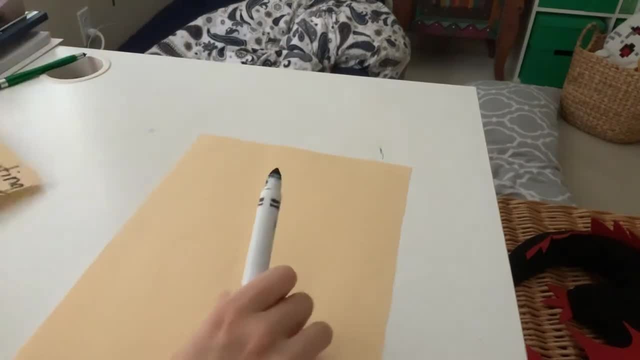 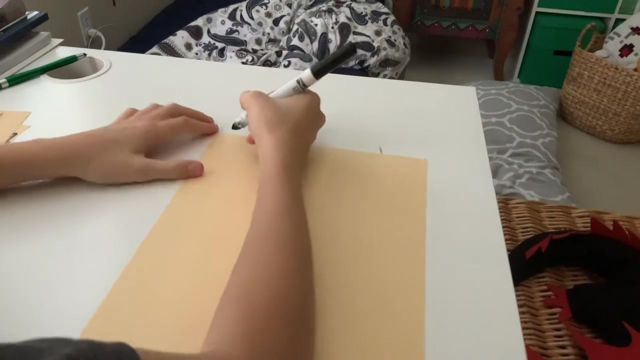 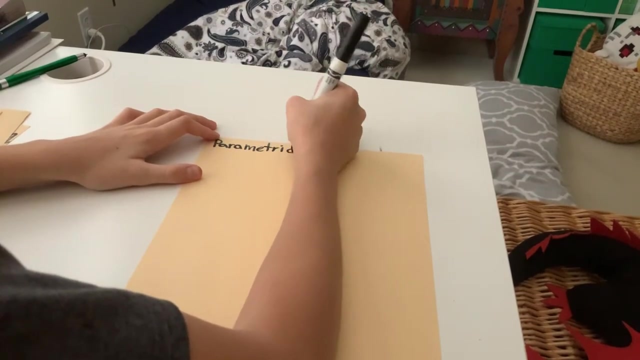 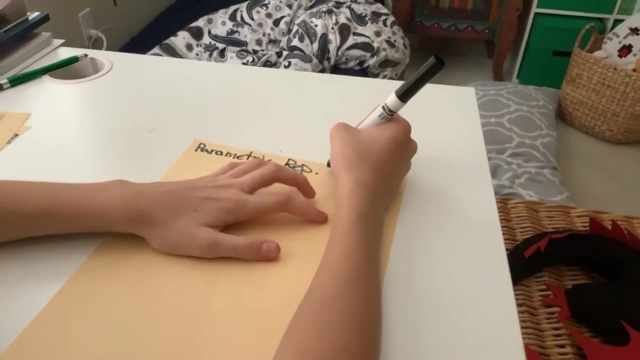 So that's why, today, we are going to be covering. We are going to be covering- I'm going to get some paper Paper's ready- I'm going to be covering parametric representations. I'm going to show them that, with the abbreviation rep. 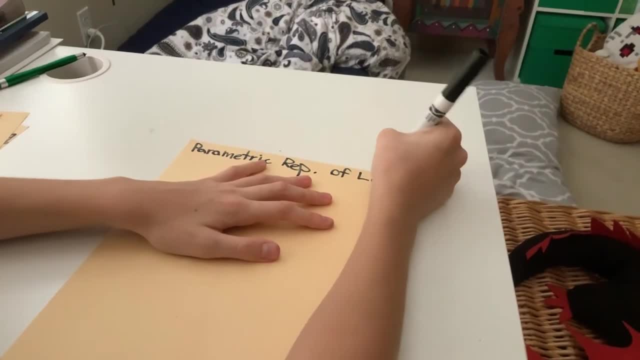 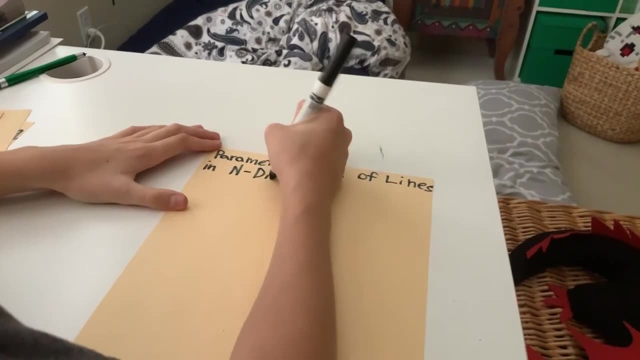 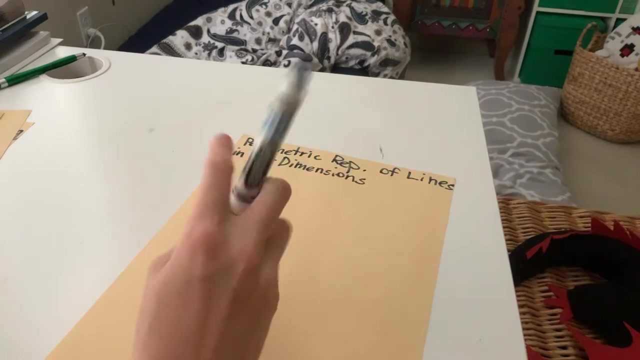 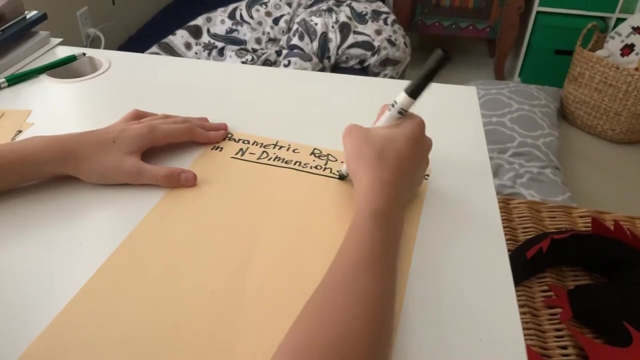 of lines in n dimensions. n meaning any dimension like one, uh uh, two dimensions, three dimensions, four dimensions, etc. n dimensions. This is the key, Okay, So why don't we start off with looking at that set definition again? 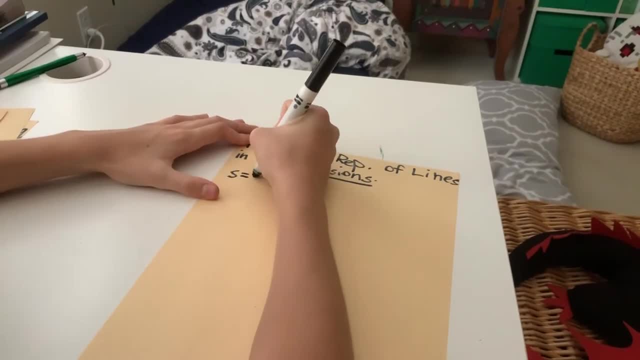 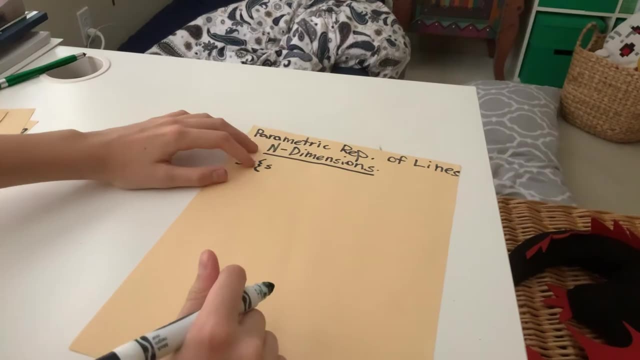 I'm going to write it down here. so we We thought of a set where Where we had any constant. In this case, I want to represent it as this, because I It's going to make sense, because obviously this stands for scalar. 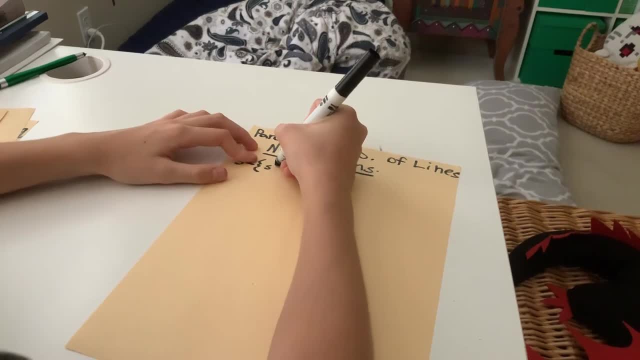 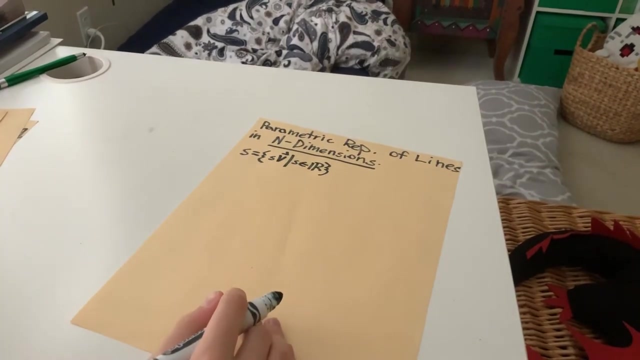 Scalar represents Scaling this vector Multiplied by a vector v Right, Such that This number, not to be confused with the set itself, is a member of the reals Right. So Let's pick out a value for. 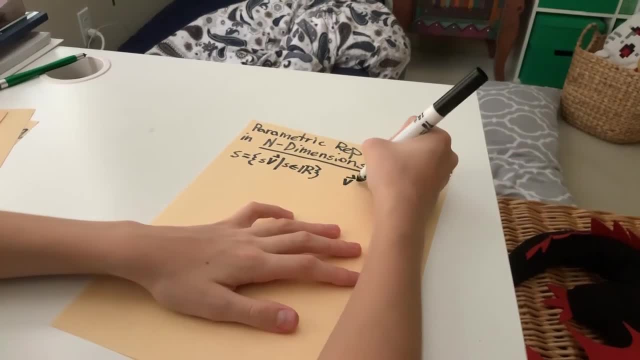 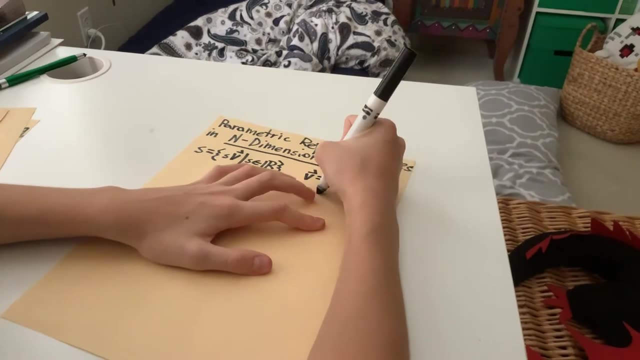 This vector v. Let's pick up, Pick out something that's not too big of a number, since I'm graphing this on paper and I don't want it to be too difficult. So let's say we have negative One Six. 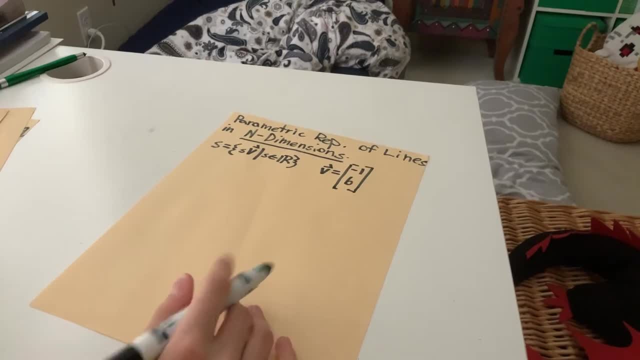 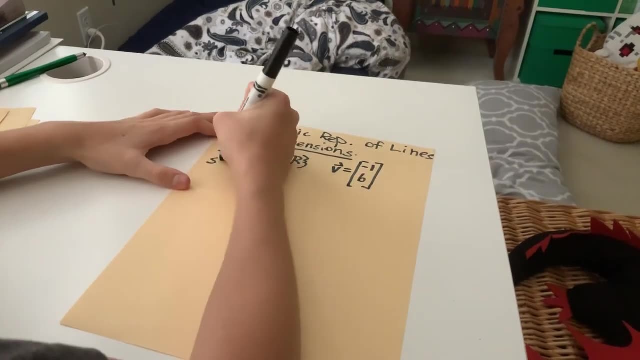 That's our vector v. So let's graph that real quick. And actually we can actually first rewrite this set definition quickly, since we've picked up, Picked out a vector For vector v in this case. So Some scalar Times: vector. 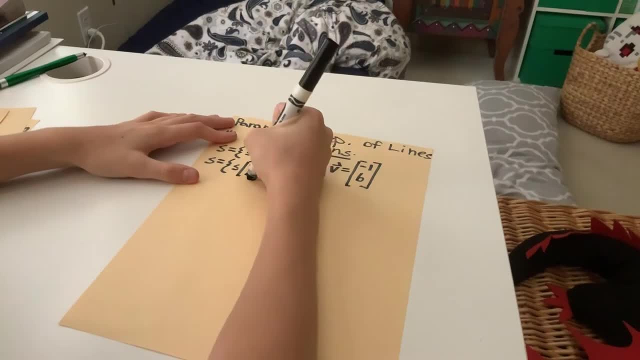 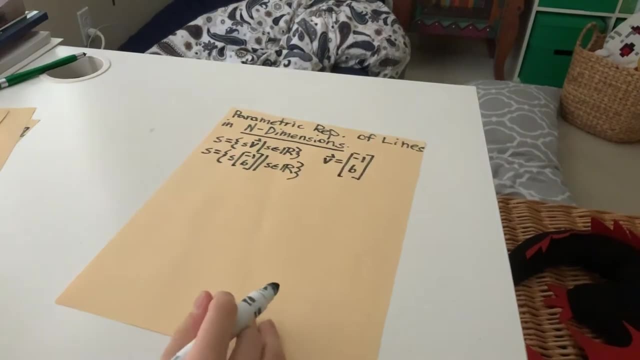 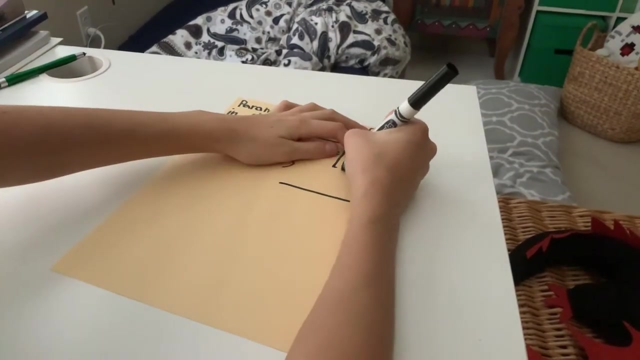 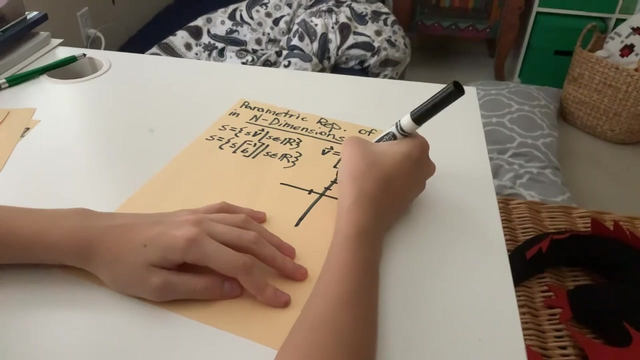 Negative one, Six, Such that Scalar is a member of the reals right. Right, Okay, So we've rewritten it in such a way, So let's graph it So: negative one, And then one, Two, Three. 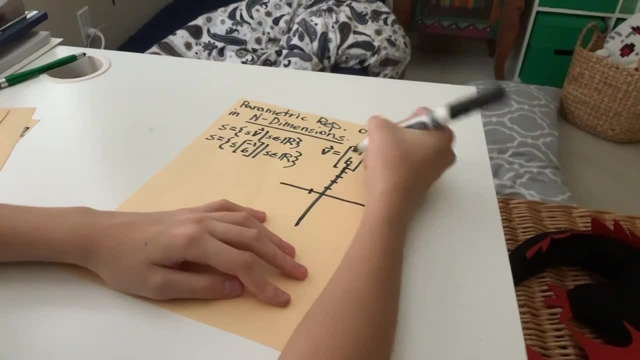 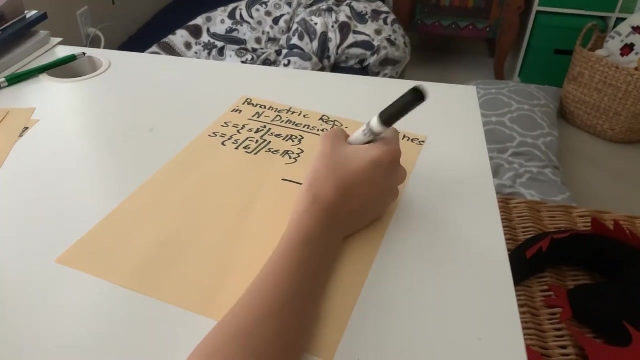 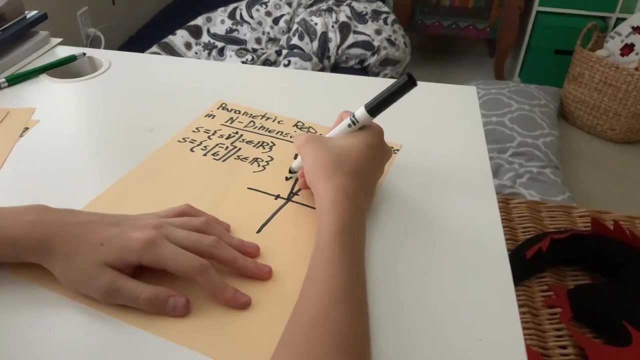 Four, Five, Six. So That is our position. vector Right: This And the head of this vector Or this line. This arrow Represents the position or the magnitude of this vector here. So this is our vector V. 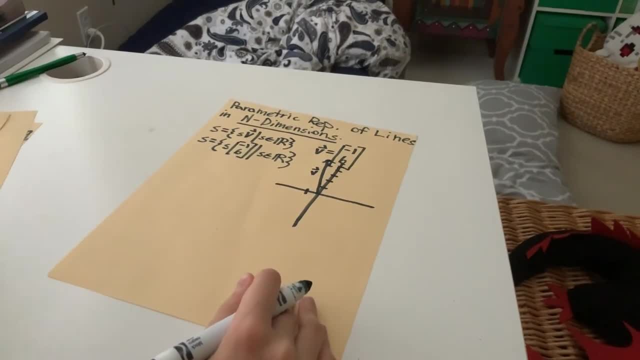 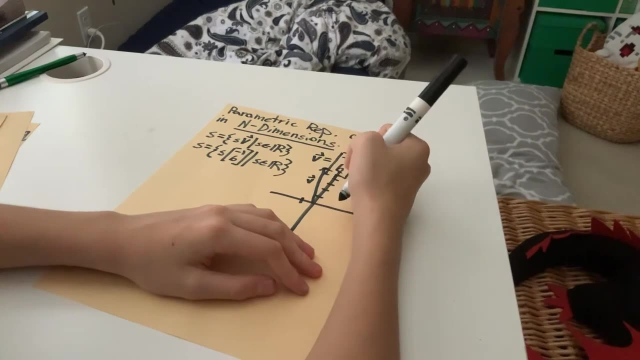 Right. And now what if we Scale this? Uh, Scale this by any Scalar s Right, So We could scale it by two. We can. I've, And I discussed this in the last video, So I. 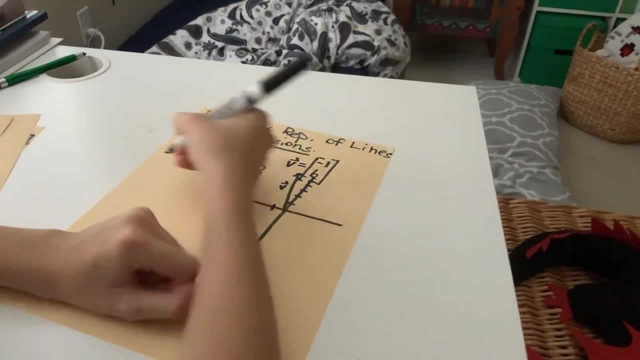 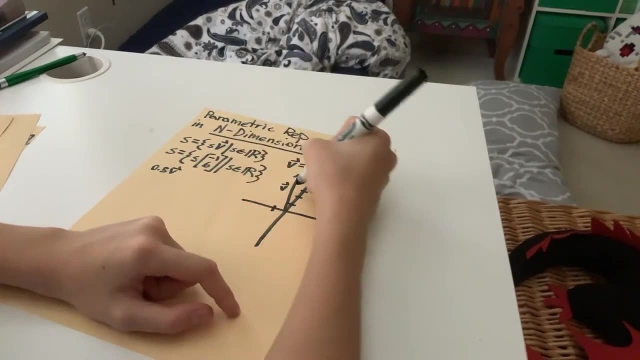 The previous video, So I recommend checking that out. I'm not gonna Go into too much detail, But Let's, for example, scale it by 0.5.. 0.5 times v, Right? So that's just half of all the coordinates here. 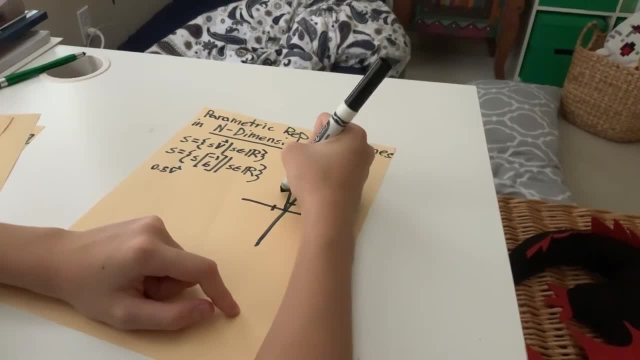 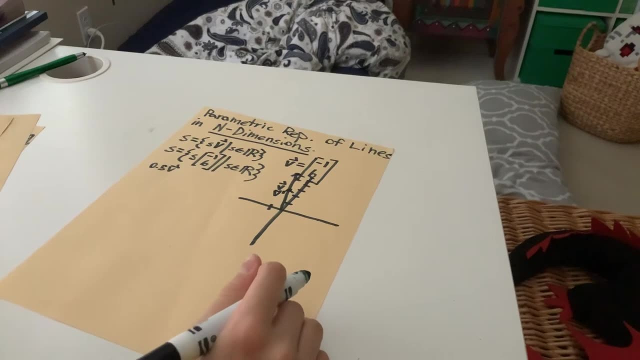 And that would end up somewhere in the middle here. Right, That would be our. You know, That would be our v prime. Right, It went through some transformation And I'll get to that later on. Alright, So that's just a brief example. 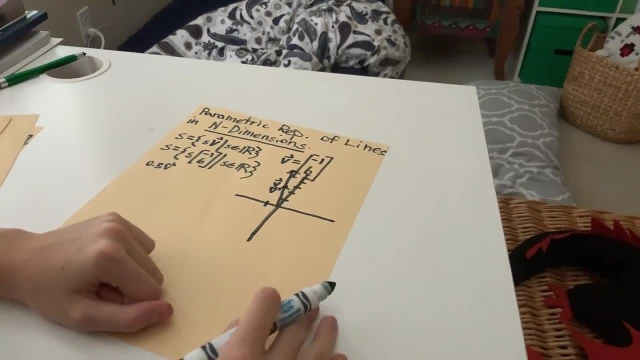 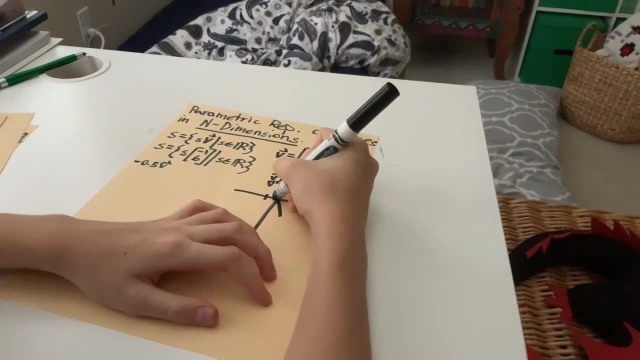 So now we, We could, Uh, Multiply that by a negative sign as well, Right, And that would just Make it collinear with, That would just make it collinear with This line here, Right, And that would be. 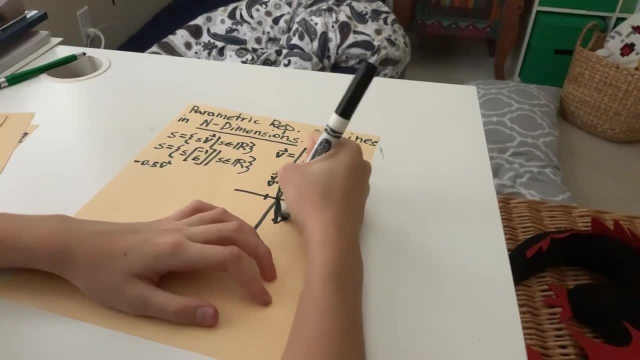 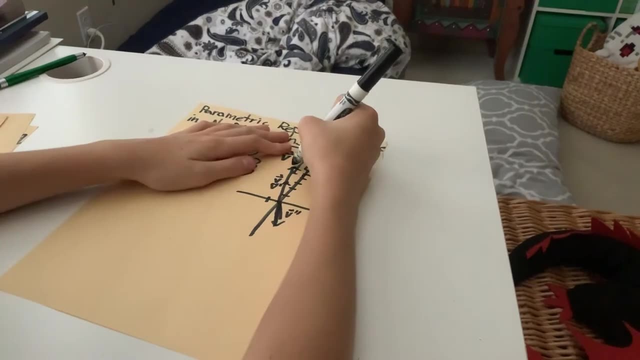 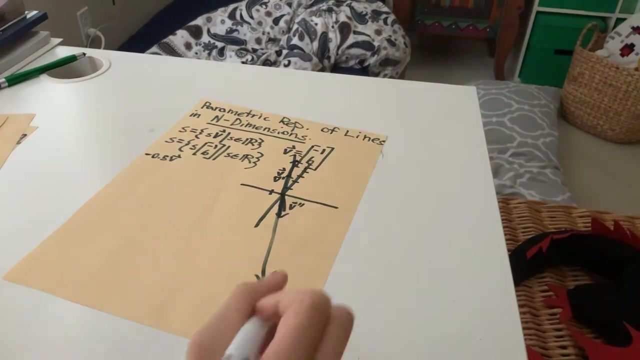 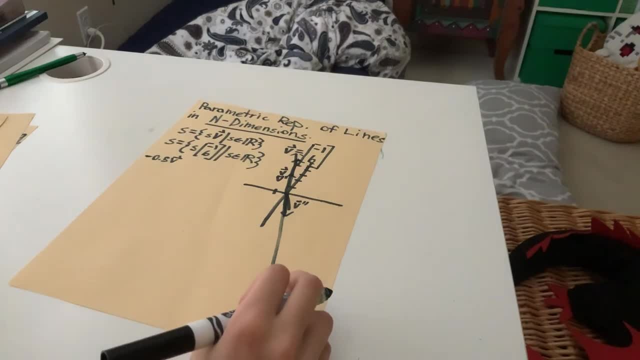 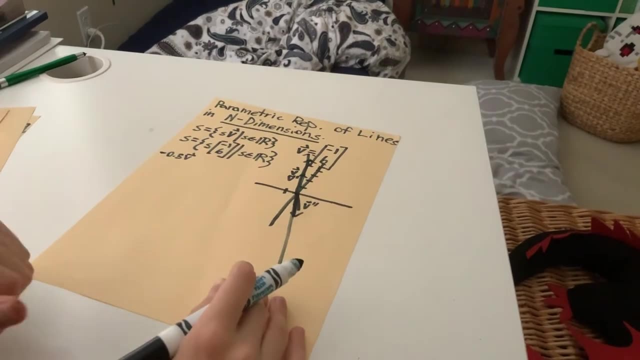 A line And this line graphs all Uh, Uh. This line goes out infinitely, So on, so forth. Right, And that gives you all the V. Uh, That gives you all the solutions, The prime number, Or sorry? 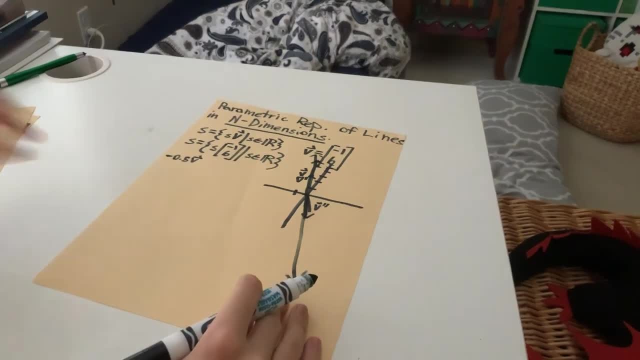 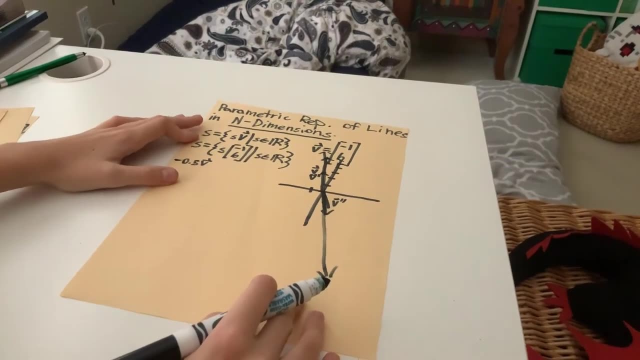 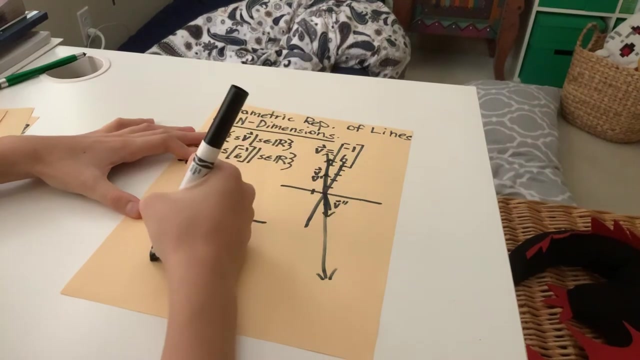 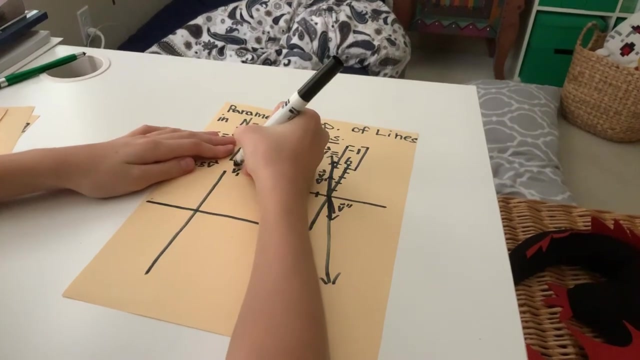 The v primes, Every v primes of this basis, V. a few more complicated topics here. Six minutes got it, So let's start off, in this case, by graphing something. We're going to graph two new points: v1 and v2.. 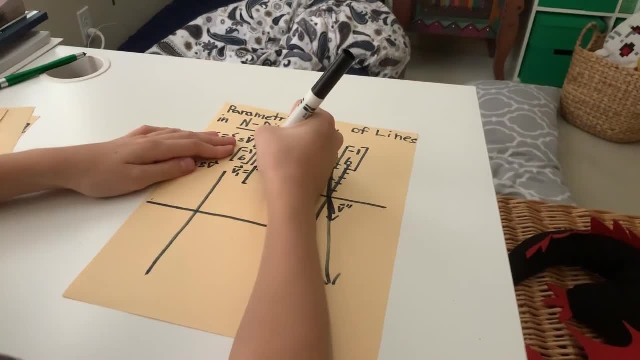 So let's set v1 equal to 4,, negative 2.. Okay, so 1,, 2,, 3,, 4.. 1, 2.. So this is our v1, vector: 1.. Then v2.. 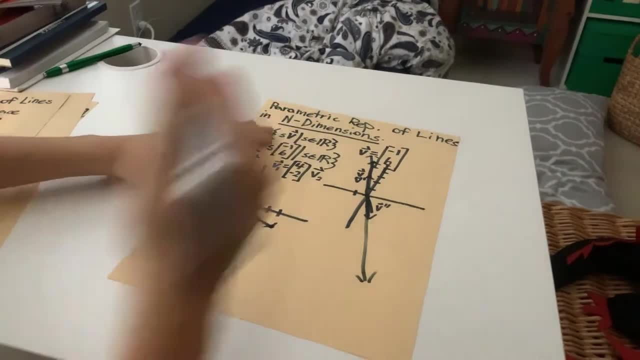 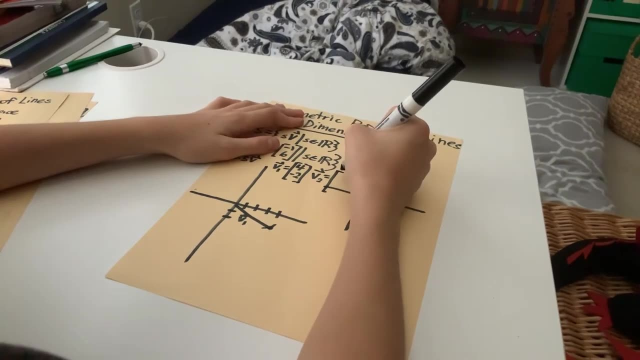 I'm just going to position this a little better. v2 is equivalent to: I don't know, and by the way, we're starting this all from standard position or from 0, 0. Let's say 3, positive 2.. So 3 and then up 2.. 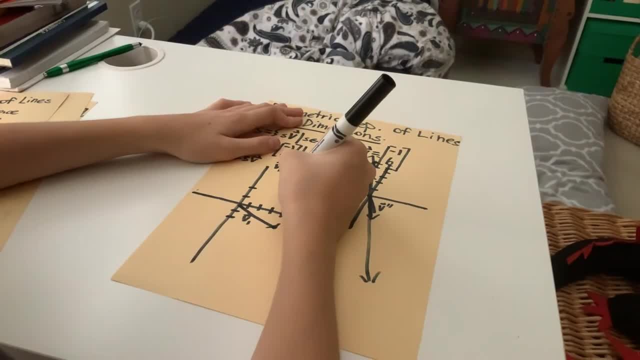 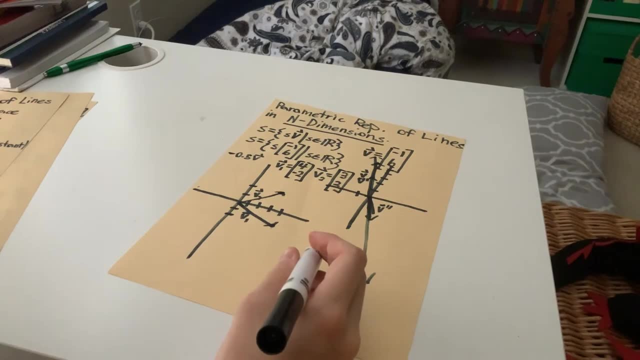 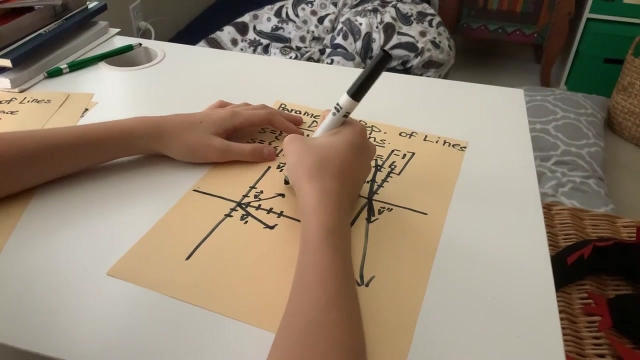 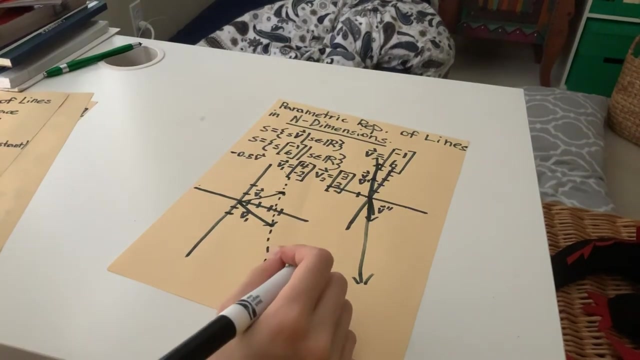 All right, and that's our v2.. And what I'm trying to say is how could we describe a line, a secant line, that passes through both of these points? right, Just like so? How could we define such a line through our definition of sets? right, And normally, what you would? 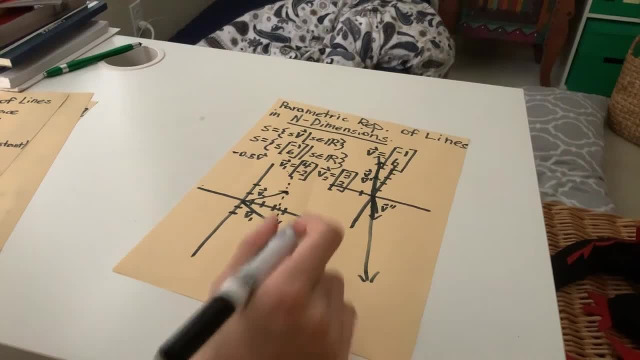 do in Algebra 1 or Algebra 2 is you would, just you would line these, the coordinate points of this up, and find the slope, and then substitute that in: et cetera, et cetera, And that would be easy, fine and dandy, right. But today, 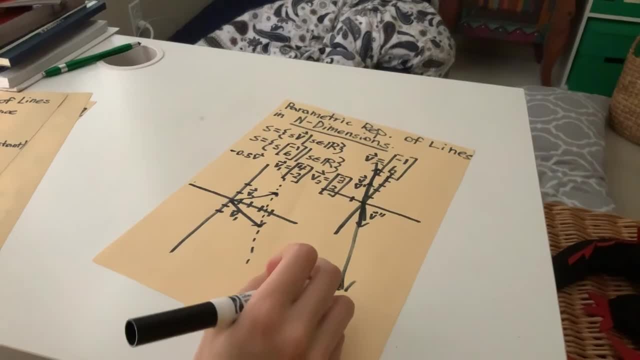 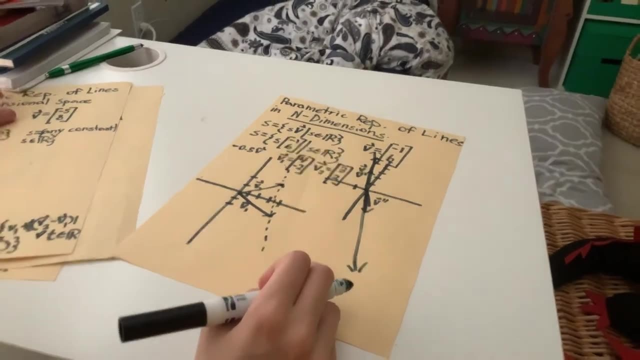 we're working with set definitions, right, So we're not going to worry about that for the time being, even though it seems easier. But in essence, you can't apply that in three dimensions or four dimensions or even five dimensions of space, right? So we can start. 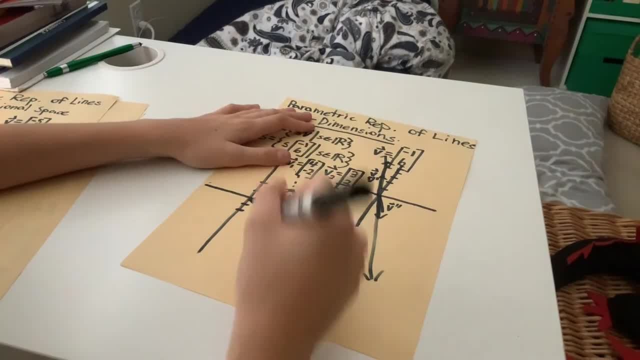 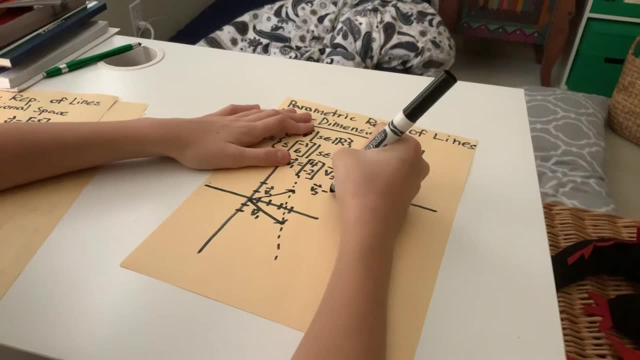 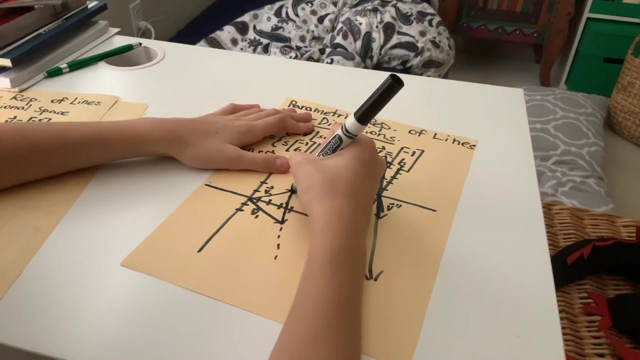 off by, you know, finding the difference of any of these two points, right? So let's say, if we did v2 minus v1, that would give us- and I described this in more detail last time, that would give us this over here, right? The difference, like the difference, what is left over this? 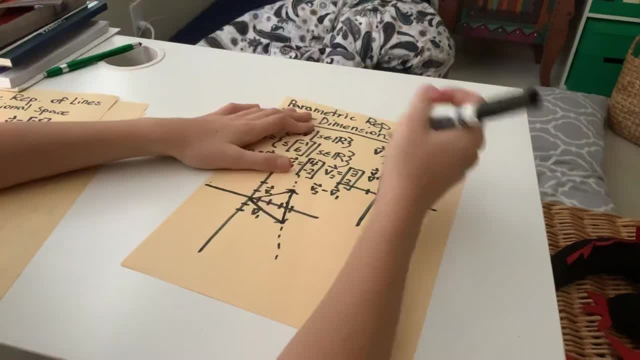 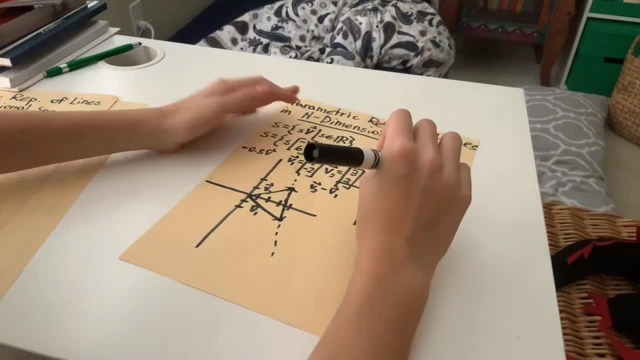 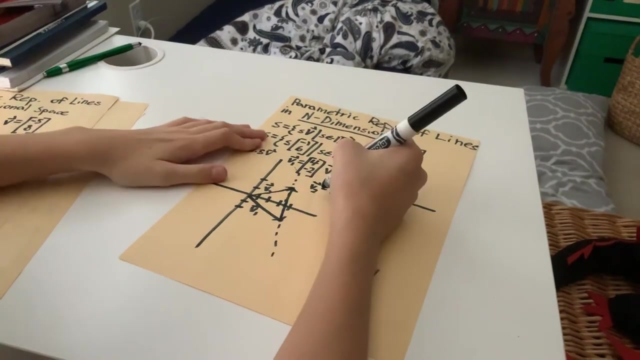 is the vector that's left over after this difference occurs, right, And it actually might be greater, right, Because we have a negative anyway, I'm not going to get to that. We went to the difference of vectors in the past, So yeah, So we can start off by this, And again we've since. 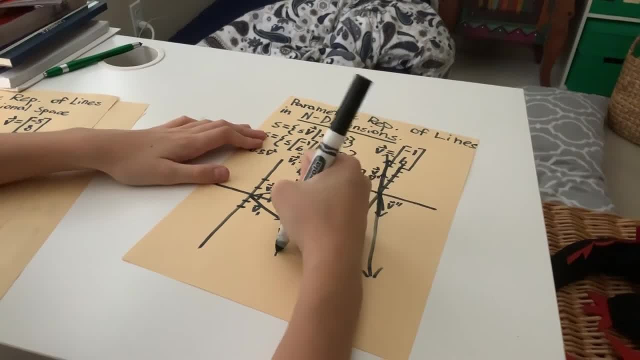 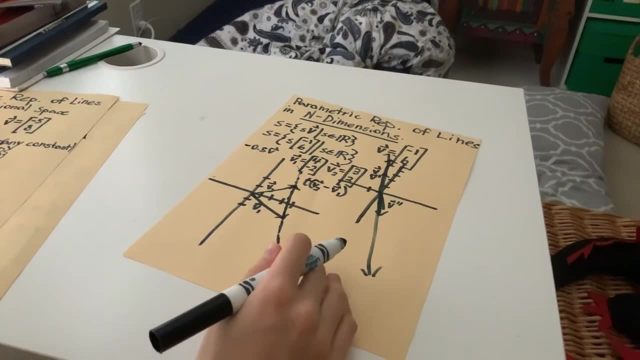 we've gone to this. we've gone to vector that's aligned with this line here, And all we have to do now is scale this by some parameter t, some random parameter t, right Or s? we could use any value, but I'm trying, as I was trying, to look familiar from when you. 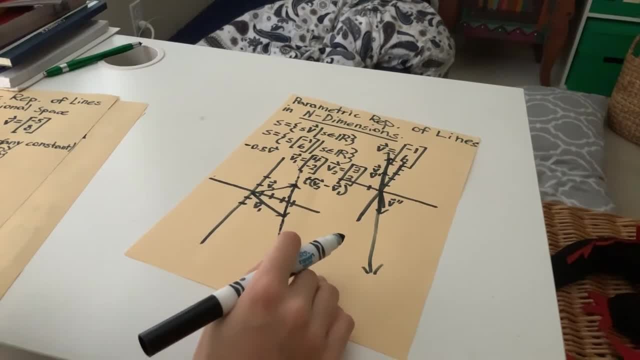 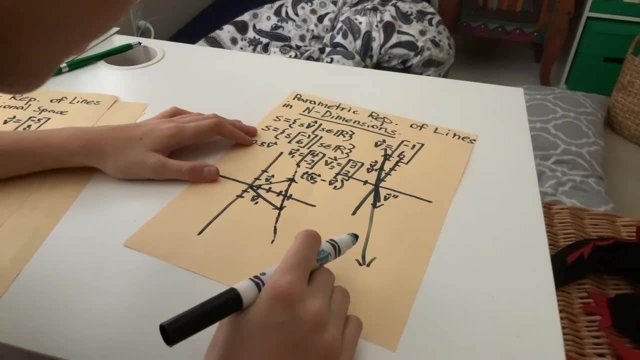 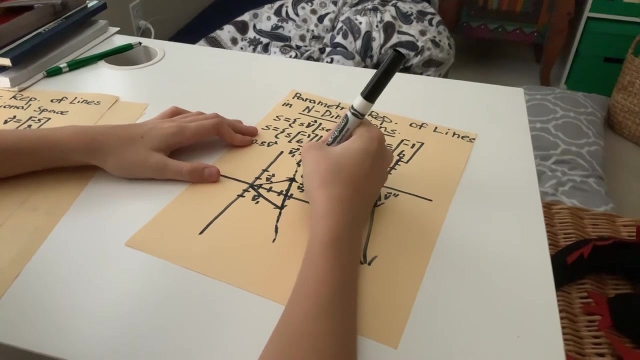 learned parameters where t can be any scalar constant, some random scalar constant, right, And this seems like it's all fine and dandy, right. This seems to work. But in reality, if you were to plot the same, the same vector or the same vector, that is the difference of these two vectors. if you 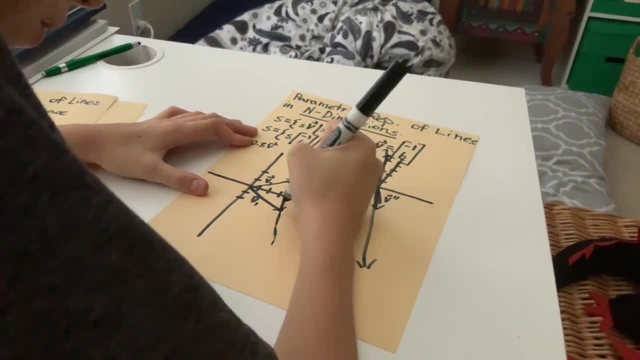 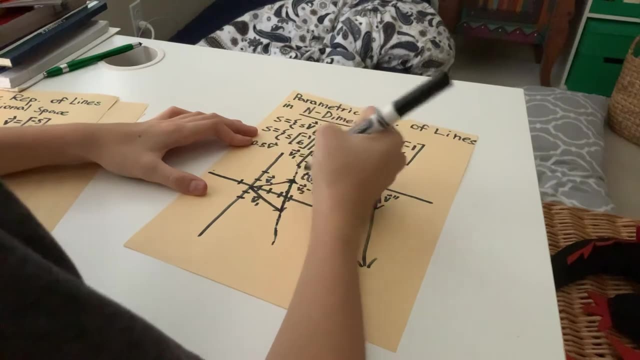 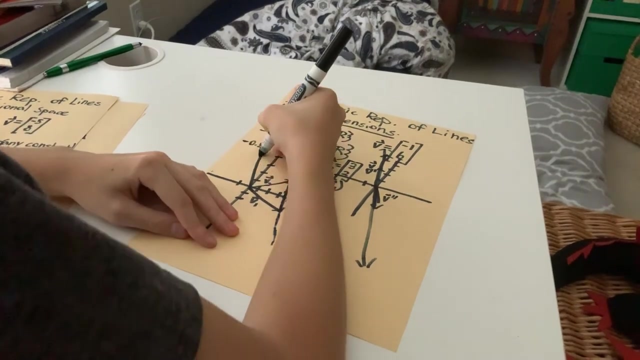 were to plot that here. so let's see where that goes. So it starts here, moves one, so that would be. so it would move back one, It would go at four, So that would be this guy. Alright, I scaled that up a bit, but it's basically what it. 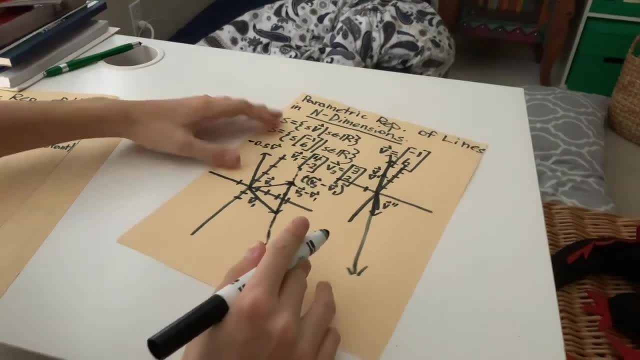 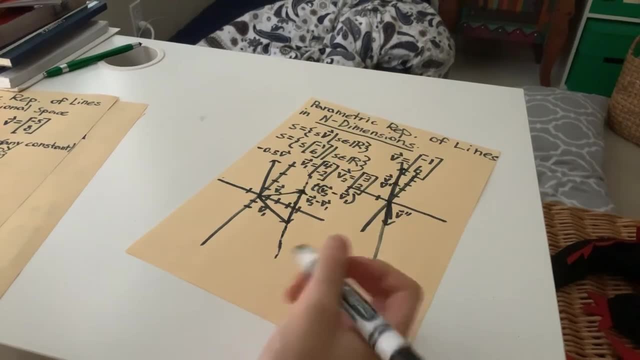 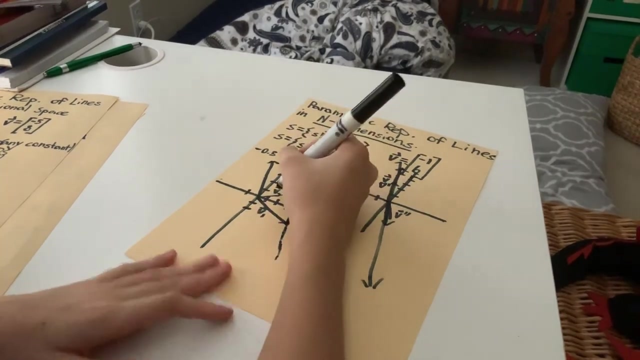 is right. Um, so this would. this is obviously an equivalent way of defining the difference of these two vectors here. right, But obviously this may be a parallel line definition here if you multiply this by any parameter. We want a definition for this line, right. 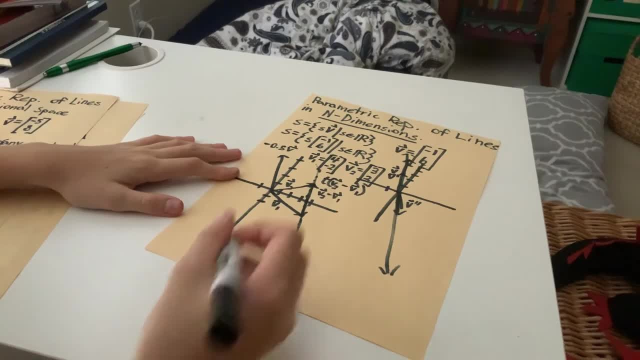 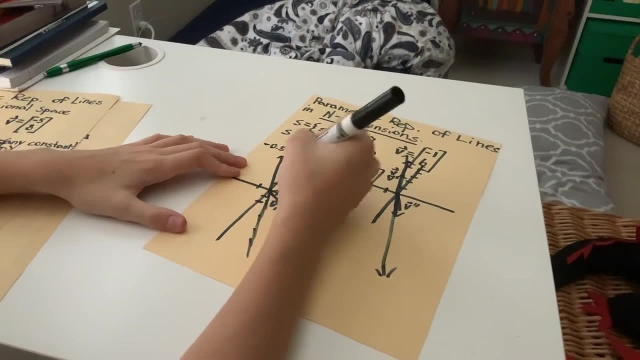 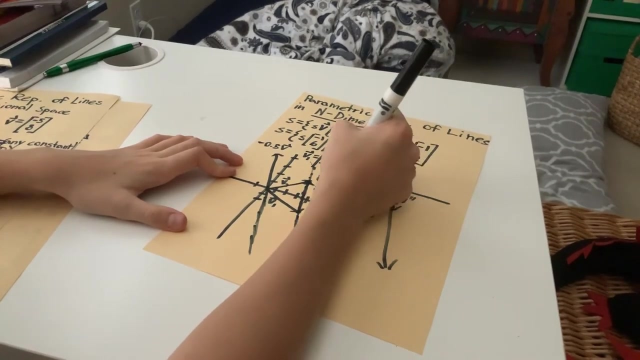 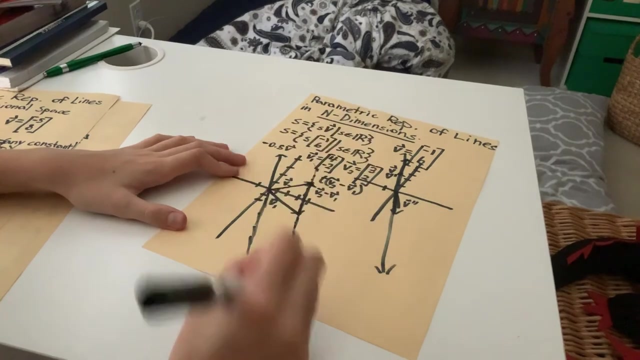 So the solution to this would be by adding either vector v2 or v1, since this is directly parallel and it's from the standard position. So, as a result, adding this to any of these scaled points with regards to this vector here that you get over here, you get some point on this line, right? 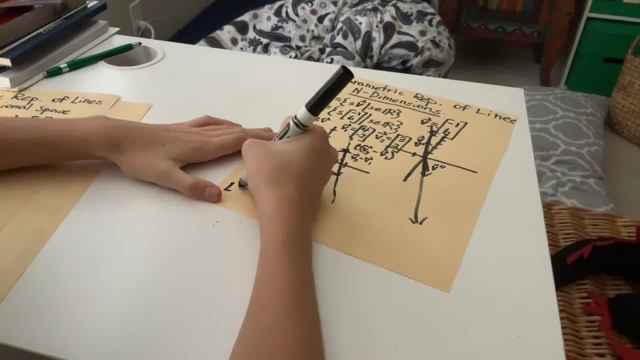 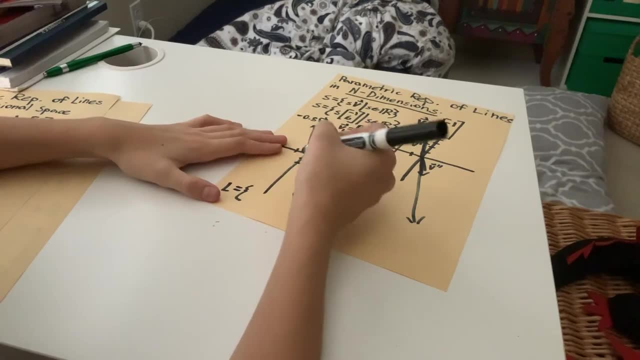 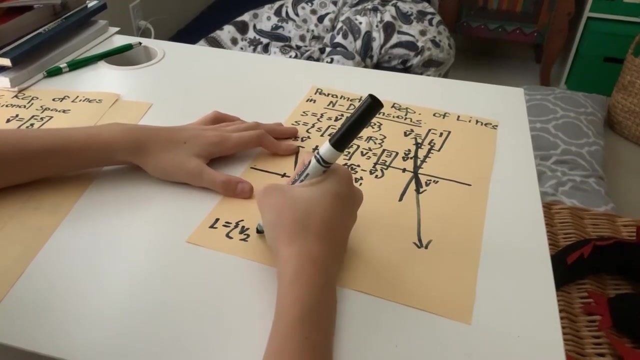 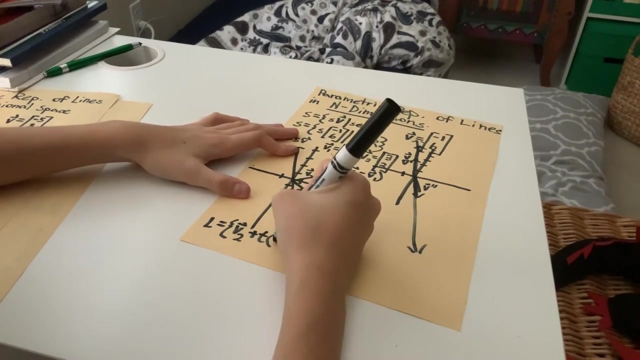 So let's rewrite this now. So now let's write L for line, I guess, and then set our parameters here, And then here's one of the options. I'll give you guys one of the options here. So let's say v2, vector 2 plus some parameter: t times the difference of v2 and v1.. 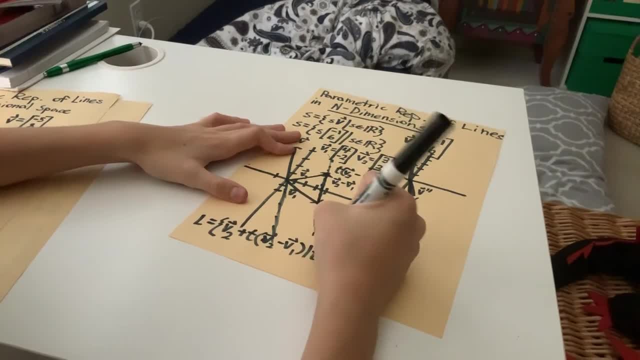 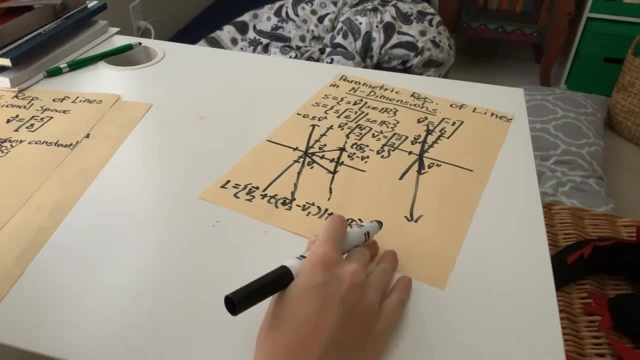 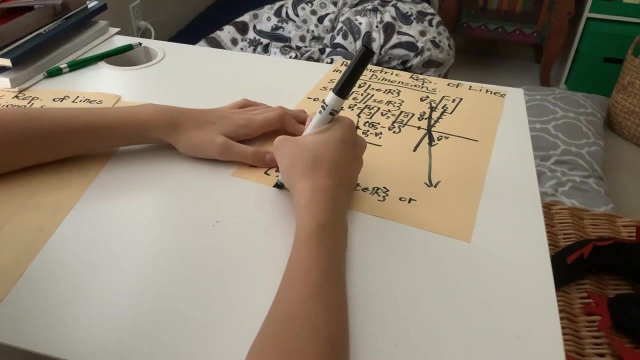 Such that this parameter t is a member of the reals. Here's one of the options. right, I'm going to have to split this up into two videos. So or L is equal to v1, vector 1, plus t times v2.. 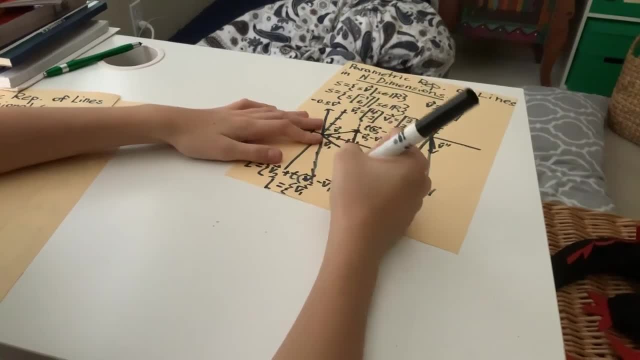 Okay, So that's one of the options. Okay, So let's write this. Okay, So I'm going to have to split this up into two times: vector 2 minus vector 1, such that t is the member of the reals. 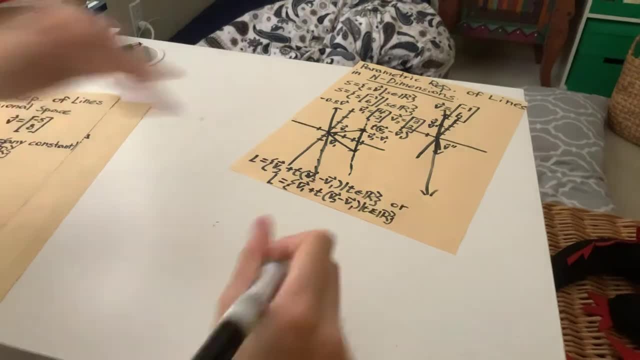 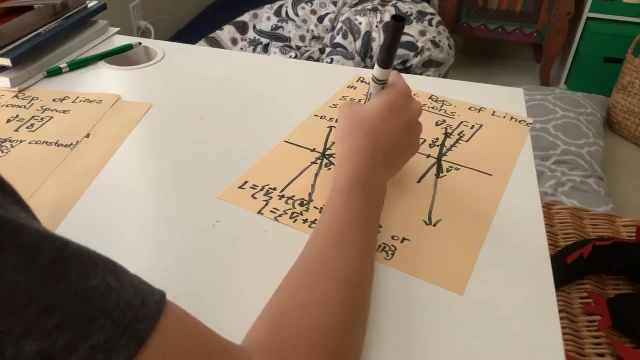 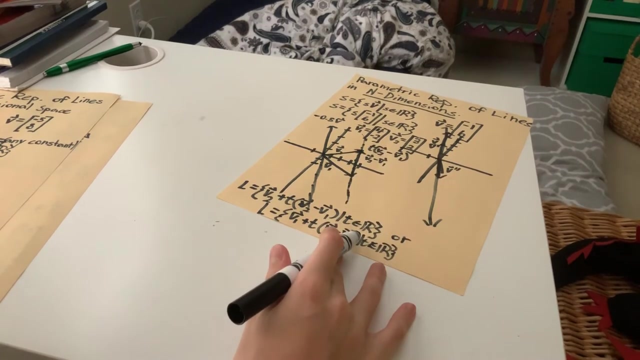 Right. So these are two equivalent ways of defining this right, Because you can tell that this is from standard position and this is the magnitude. So that just gives you any point on this line here that we want to define. So, look, we've just defined a line and this is really useful for multidimensional things. 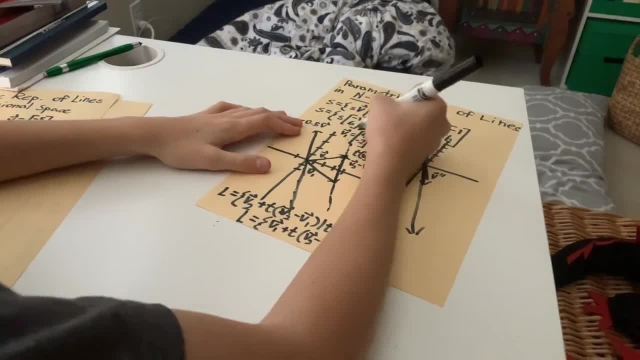 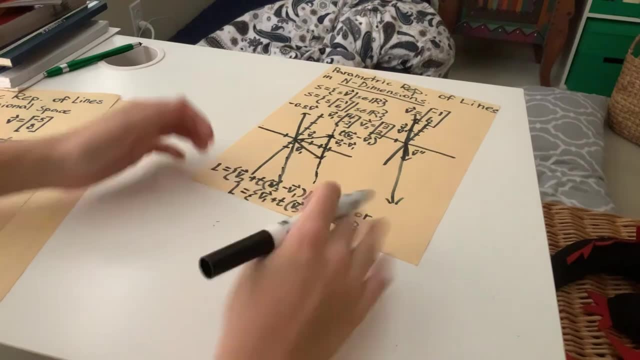 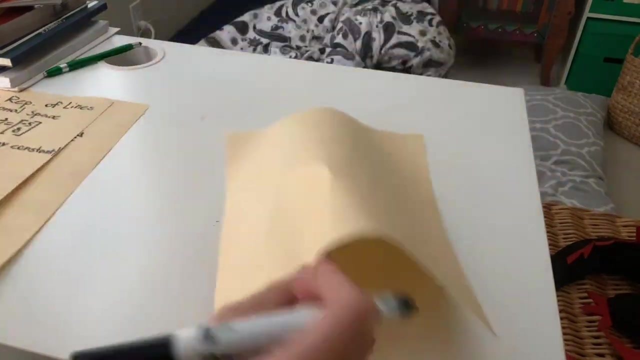 right. And now, since we have these two points already- v1 is equal to this and v2 is equal to this- we can try plugging this into this definition of a line per se. So L is equal to- and we're running out of space. here we get a new piece of paper. 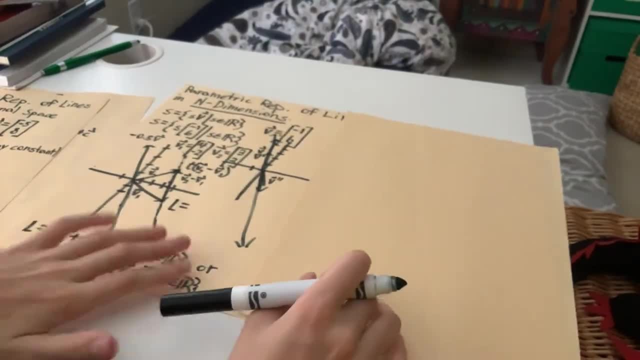 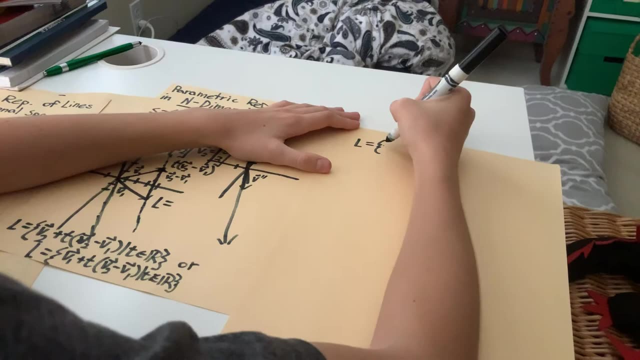 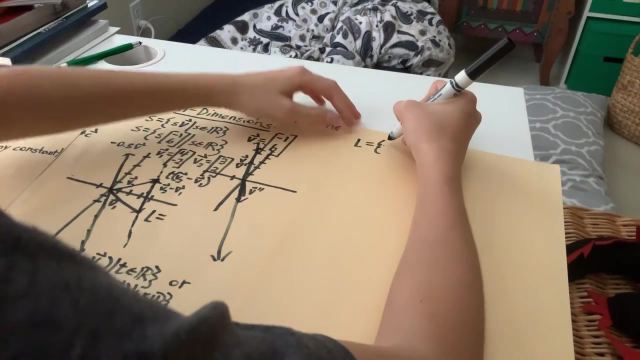 Oh, that was close. So L is equal to 4.5.. Okay, Okay, Okay, Okay, Okay, L is equal to v2.. We'll use v2 as an example here. I could use v1 as well, but I'll use v2.. 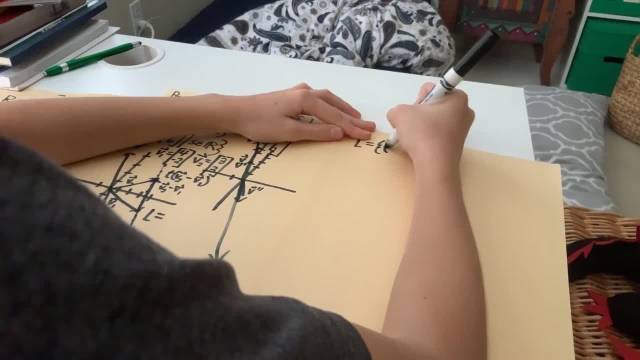 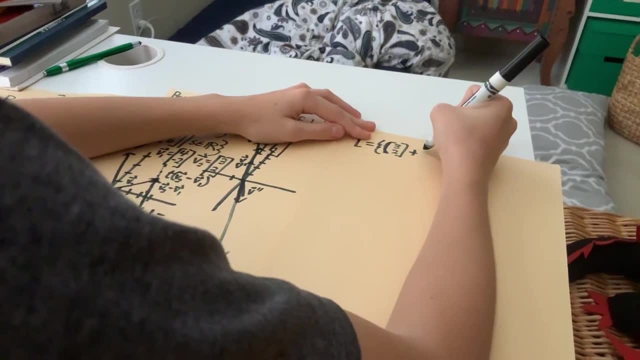 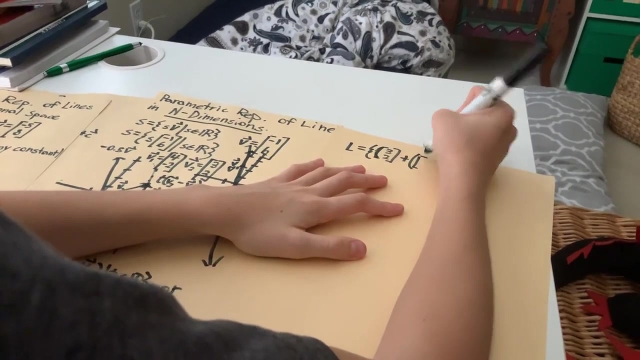 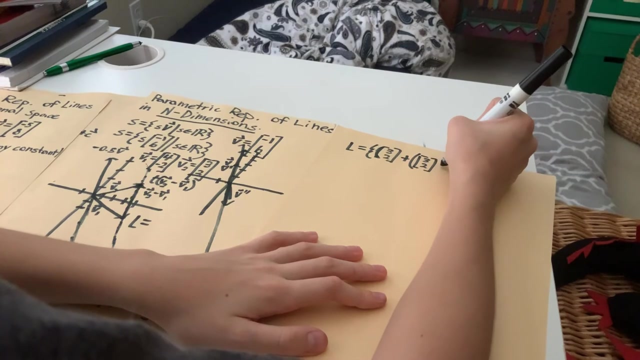 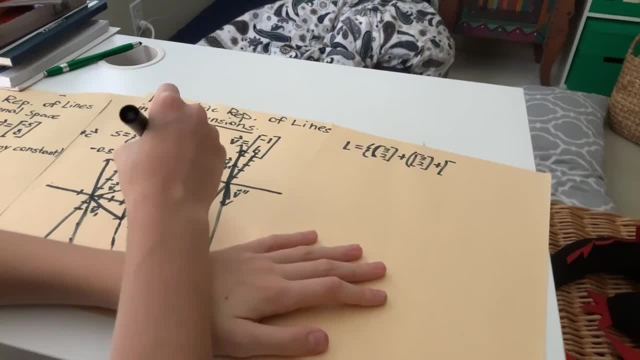 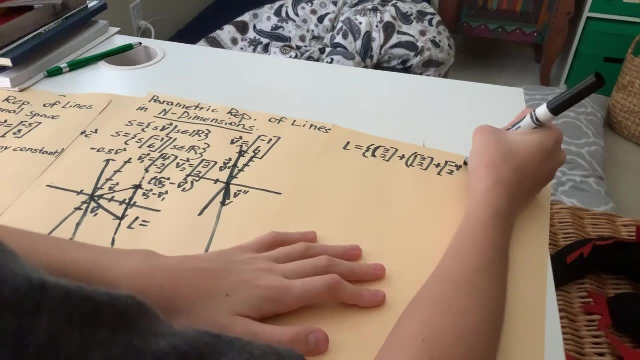 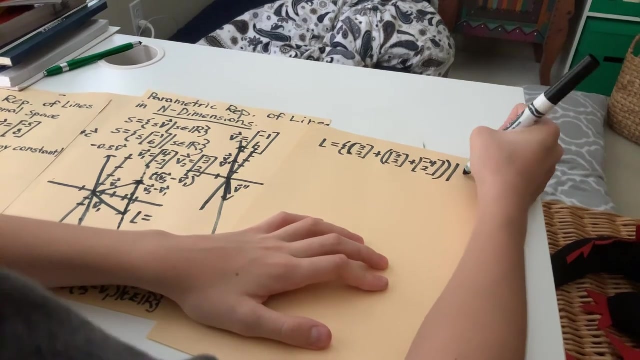 I'll, actually I'll distribute the negative 1 here, So plus. I know this is difference, but as we saw on the previous video, we could just distribute the negative 1 here. So negative 4, and 2, right, such that, oh, I forgot the parameter t. 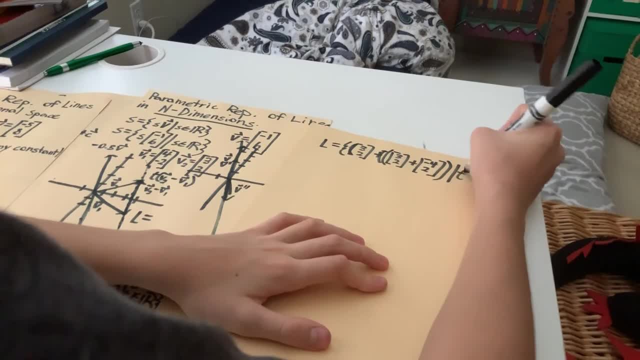 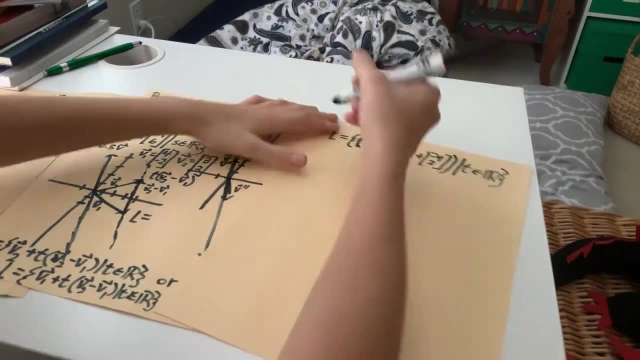 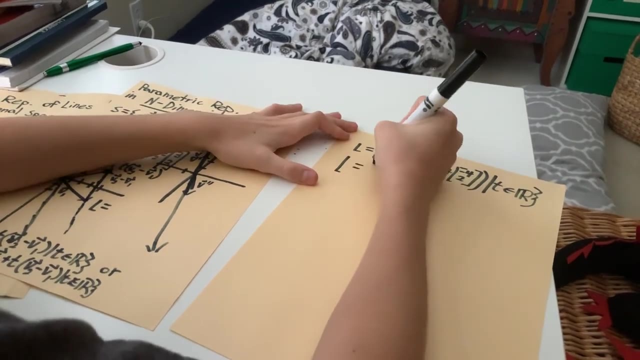 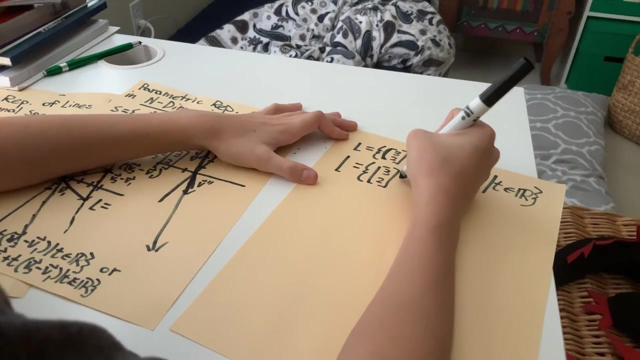 Oh, okay, parameter T, such that T is a member of the reals Yep, and that is our sub- I'm going to simplify it. just add these two together. Honestly, that's a long L, 3,, 2, plus T times. 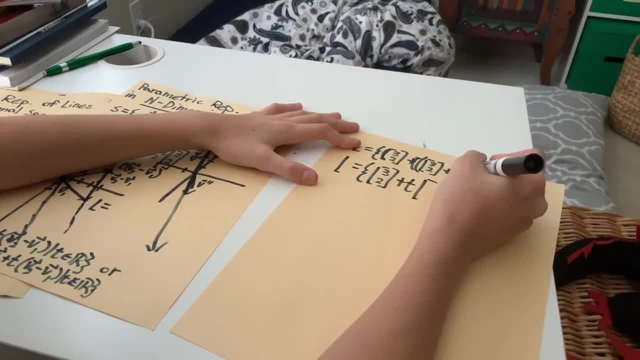 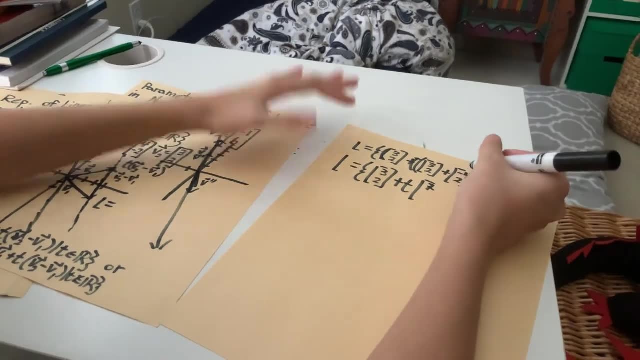 okay, so 3 minus negative 4, that's 3 plus 4, which is 7,, and then 2 plus 2, it's 4.. Oh wait, no, we're not subtracting, we're adding my bad. So this is negative 1, and. 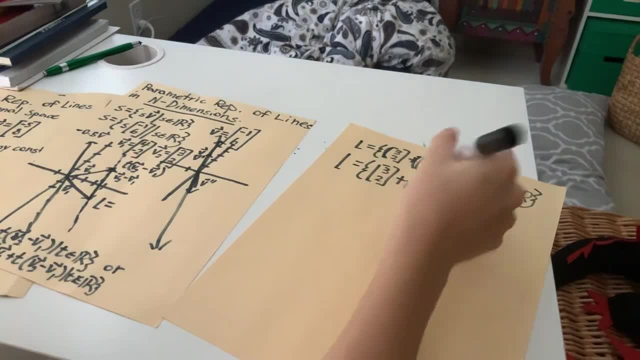 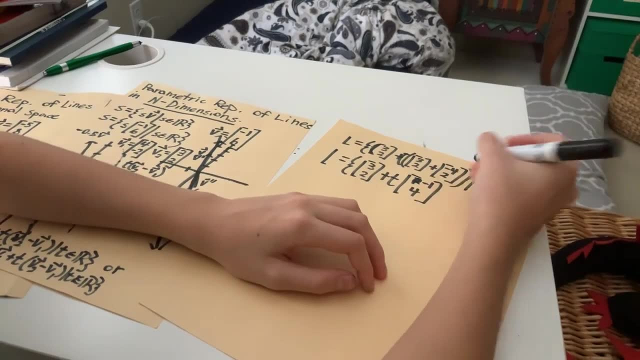 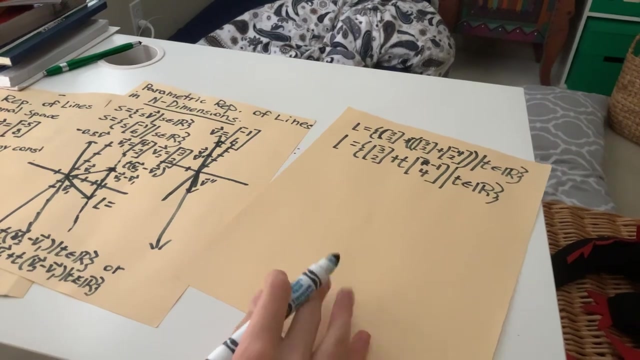 then 4,. right, Because we went to back 1, and we went up 4.. So that makes sense. Plus T times this, right. And now let me just write our- and then we just write our- T. our parameter T is a member of the reals. So you might be thinking: how do we put this? 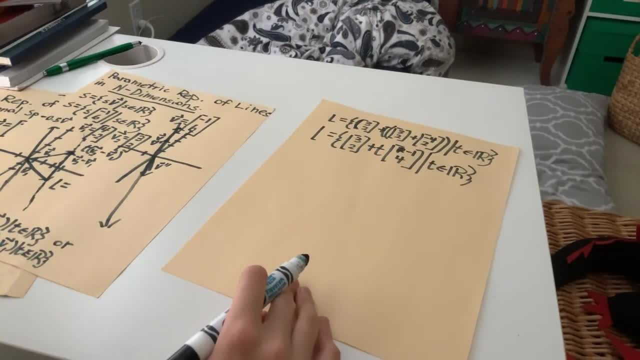 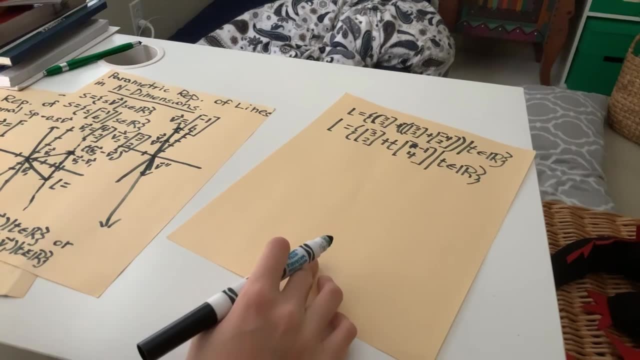 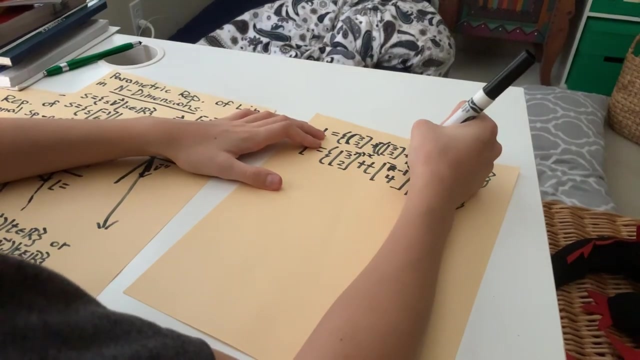 into a parametric- you know, parametric- two parametric equations, since we're dealing with two dimensions- three for three dimensions. but you get the idea. Okay, I'm going to finish this video in a bit. Well, basically, we can say that this- this is our x coordinate and. 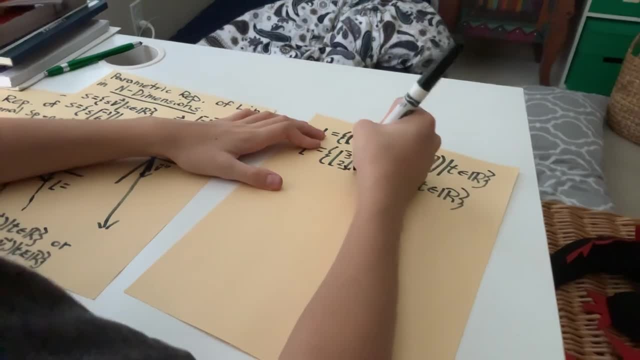 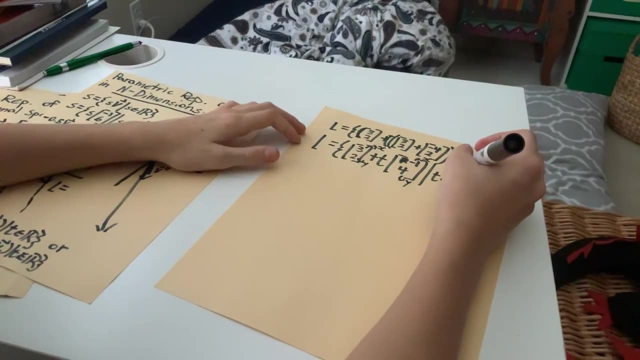 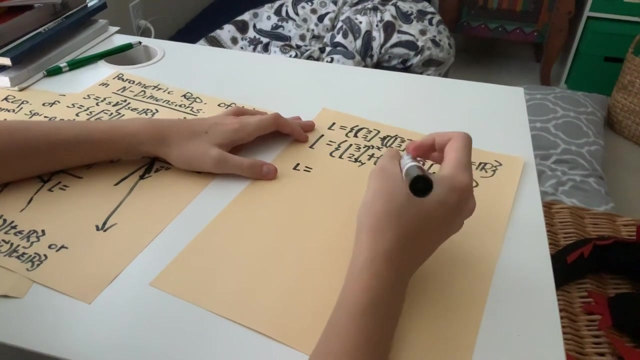 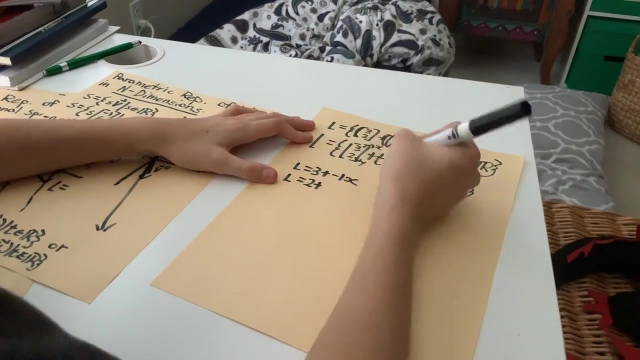 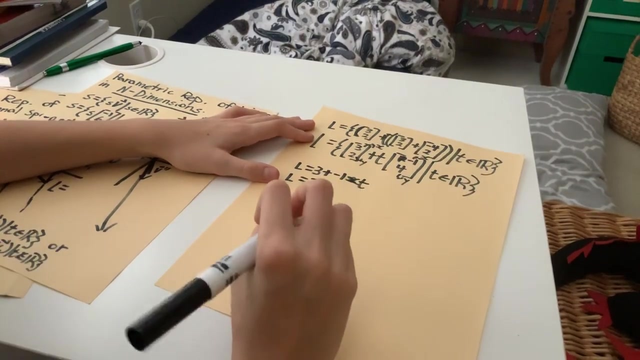 this is also our x coordinate. These are our y-components, right? So now we can say that our line can be defined using these equations. So 3,, our constant 3, plus negative 1 times x. And our second equation is 2 plus my bad, this is supposed to be t. we're thinking in terms of t, right? 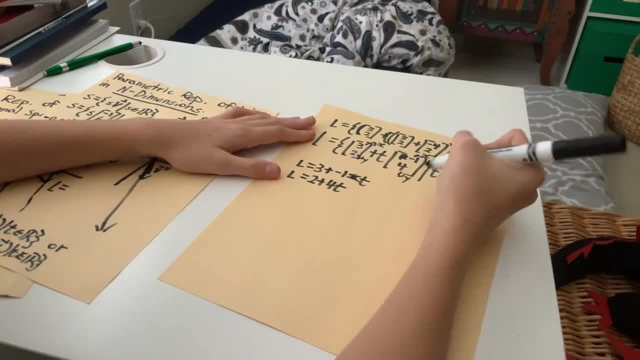 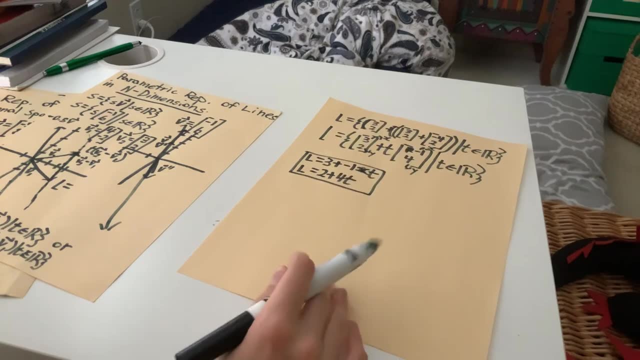 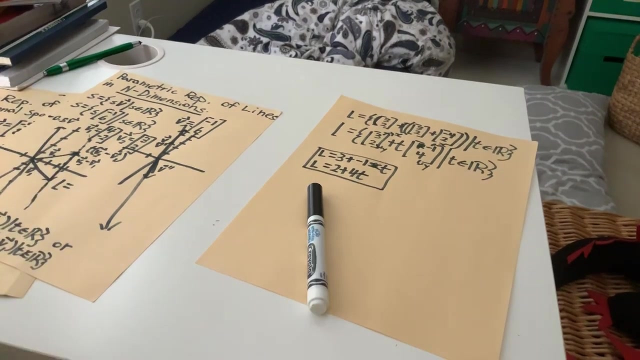 Plus 4t, And these are. this is the standard parametric equation that we've just derived from using our set definitions in linear algebra, So hopefully you guys learned something today. I hope you enjoyed the video And I'll see you in the next few videos. Bye-bye.